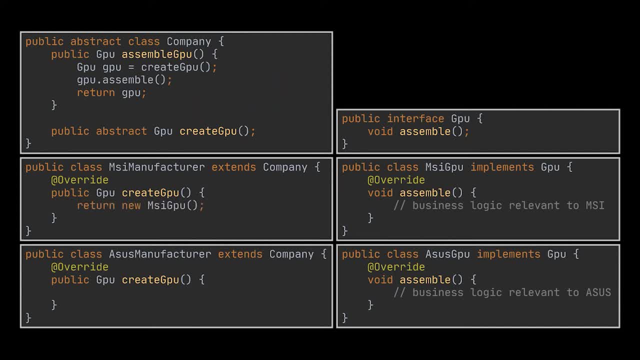 in this case. So the MSI manufacturer class will return MSI branded GPUs and the ASUS manufacturer class will return ASUS branded GPUs. Okay, until now, all we did was apply the factory method pattern and our code is clean and nice. but when does the abstract factory come into play? 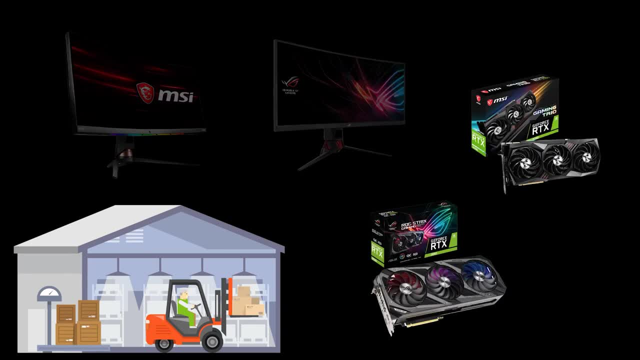 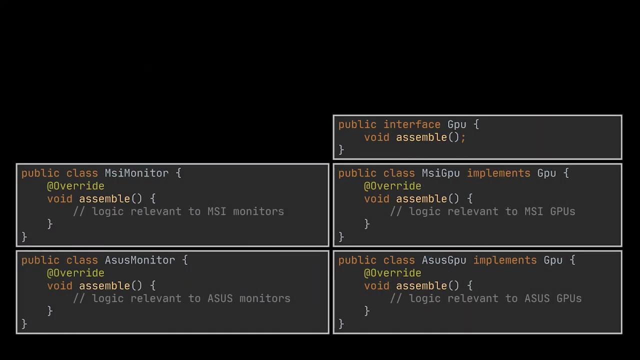 When should we use it? Well, imagine that your company started to manufacture monitors on top of GPUs, and these monitors can also be MSI branded or ASUS branded. Let's try to integrate this requirement in the code we just implemented. The first thing most people will start by doing is create a different class for each. 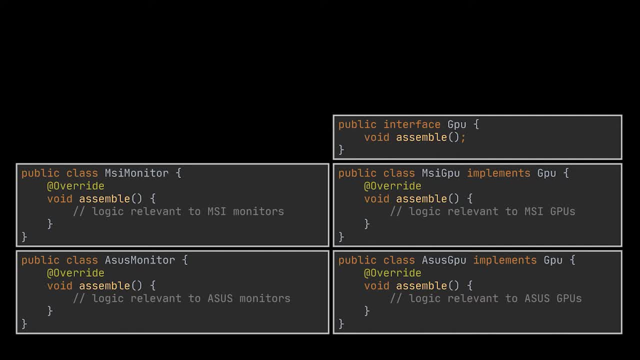 concrete component or product we have. In this example we will have the MSI GPU, the ASUS GPU, the MSI monitor and the ASUS monitor classes. Then rename the GPU interface to something broader like component and then let each different concrete product implement this interface. 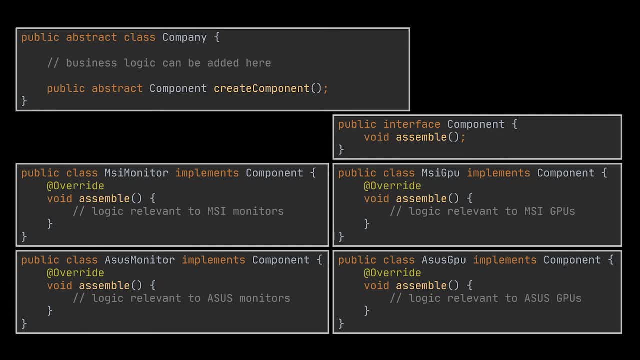 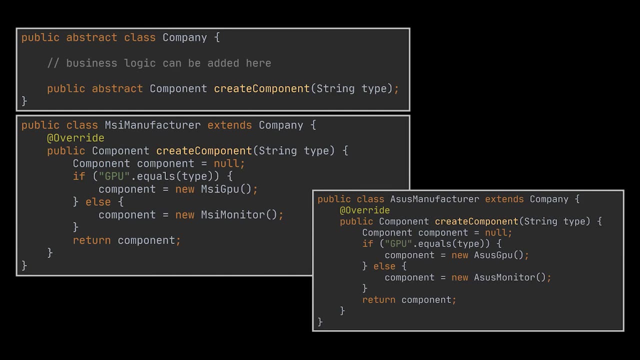 Now all that is left to do is rename the factory method inside our company class from create GPU to create component And pass the type of product we need to this method. Consequently, in our concrete creators or manufacturer classes, and with the help of the type we just added, we will be able to return the correct product requested by the 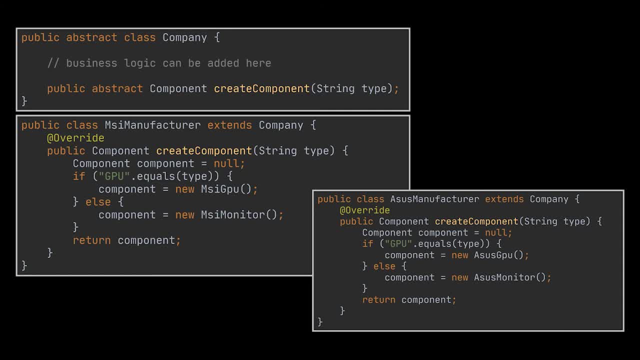 user. The modifications we just did will lead to a working solution and will help us expand our company. However, the resulting code, you see, may change. when things change, like if we start handling new computer components, we're going to have to open this code and change it, and that 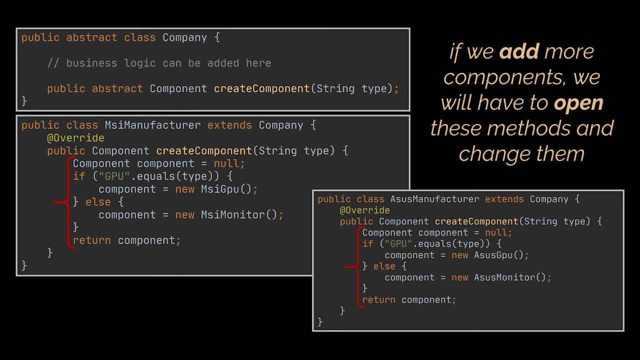 violates the open-closed principle. Now, some of you may be wondering: how did this guy manage to violate the open-closed principle even though he was applying the factory method pattern? Well, you see, in this particular example, a single factory is not enough, and that is. 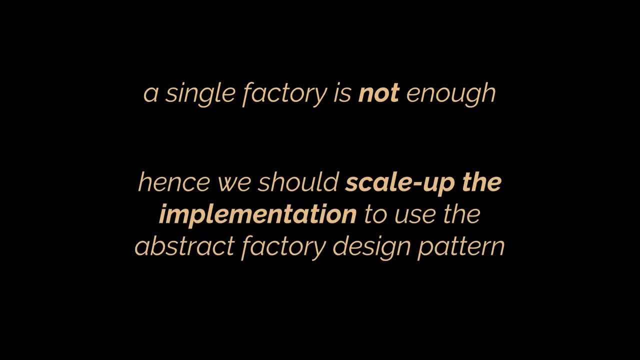 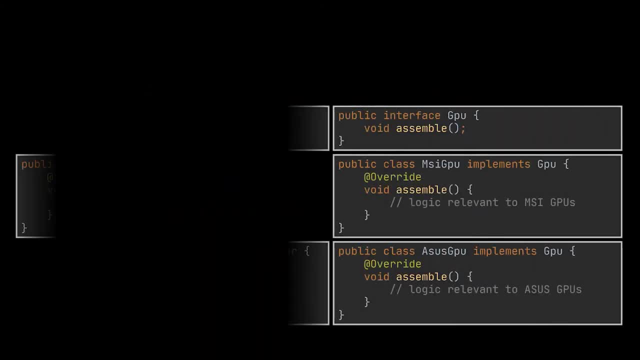 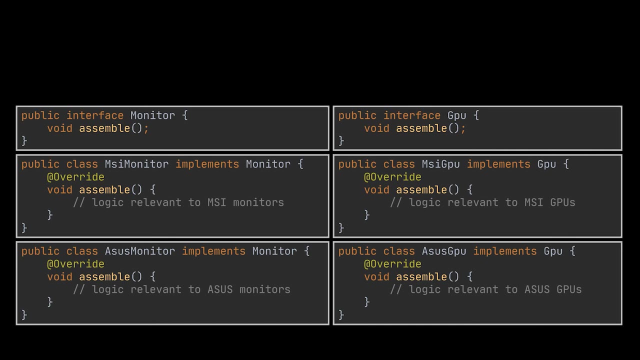 where you should start thinking about calling up your implementation from the factory method pattern to the abstract factory design pattern. To do this, let's bring back our GPU interface and create a separate interface called monitor. This interface will be implemented by the ASUS monitor and MSI monitor classes. 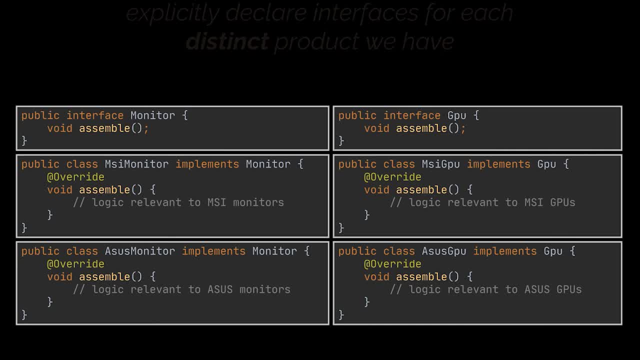 You see, the first thing the abstract factory pattern suggests is to explicitly declare interfaces for each distinct product we have and then make all variants of these products follow those interfaces. The next suggested move is to create inside our abstract factory which, in our case, will: